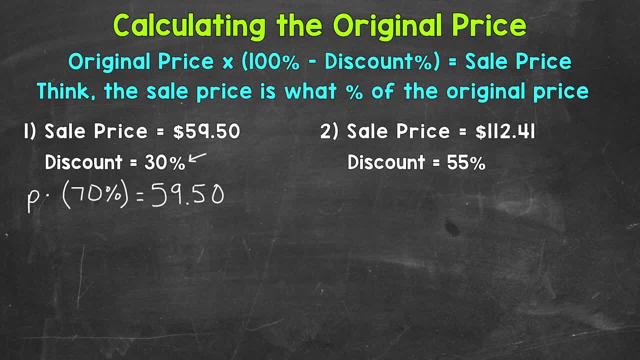 one again. we did 100% minus 30% and that gives us 70%. We are paying 70% of the original price. Now let's convert that percent to a decimal so we can move forward within our equation here. And remember: percent to decimal. move the decimal twice to the. 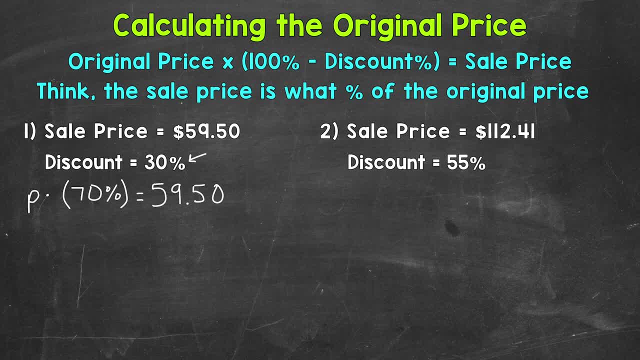 to the left. So the decimal comes at the end of 70, end of a whole number here, And we need to move it once twice to the left. So again we're converting that percent to a decimal. So let's move on here and rewrite our equation with the percent in decimal form, So we have the original. 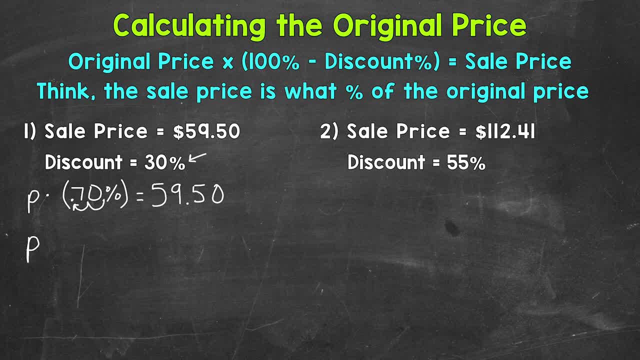 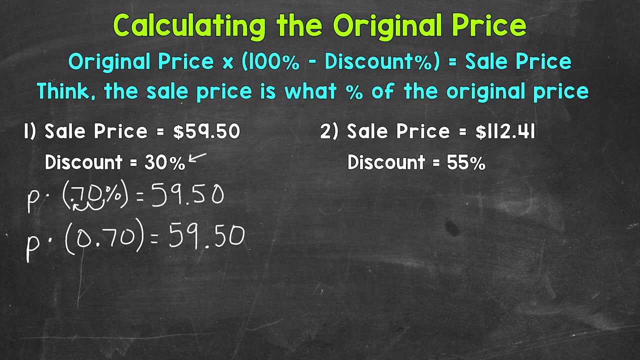 price, which is a variable of p, because it's an unknown times 70%, as a decimal is 70 hundredths And that equals our sale price of 59.50.. So we have a one step equation here. we need to isolate our variable here. So we have p times 70 hundredths, What's The opposite of. 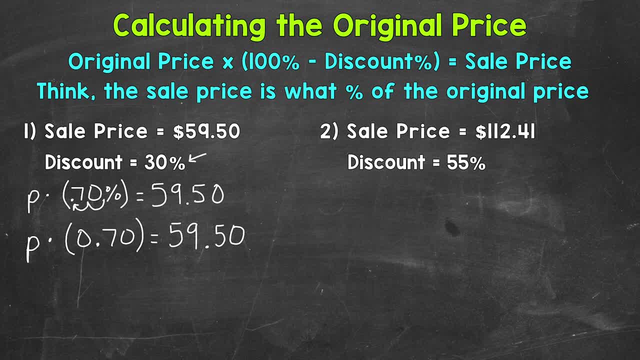 multiplication, Well, division. So we need to divide that side by 70 hundredths and that's going to cancel out our 70 hundredths and isolate our profit And that's going to get us there in a our variable. Now, whatever we do to one side, we have to do to the other in order to keep 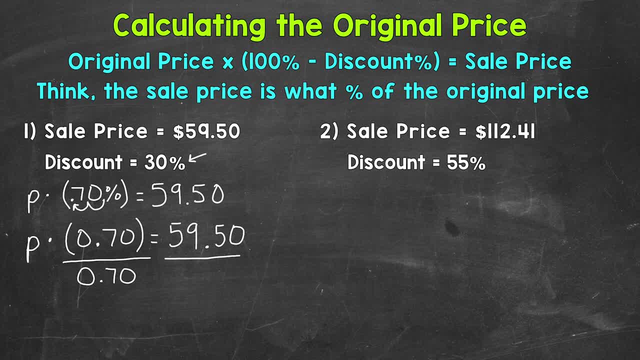 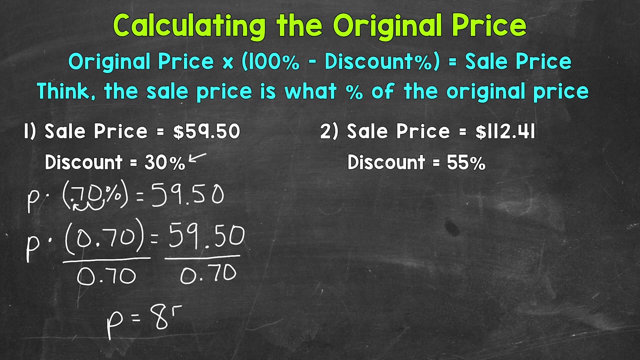 our equation balanced. So let's divide this side by 70 hundredths as well. So our variable of p, the original price, is now isolated and we can do 59.50 divided by 70 hundredths to get our original price, and that's going to give us 85 dollars. So 85 dollars is our original price. 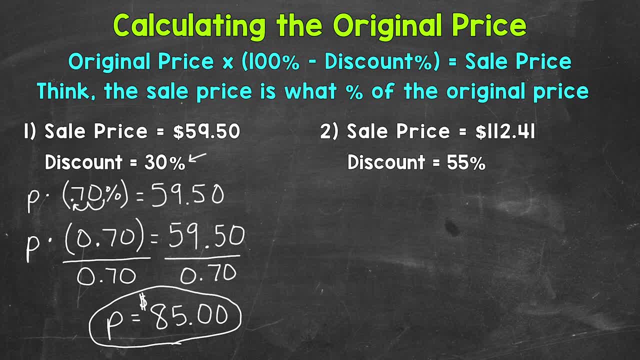 Let's move on to number two and do another example. So we have a sale price of 112 dollars and 41 cents and a discount of 55 percent. Let's find out what the original price was. So we'll set up our equation.